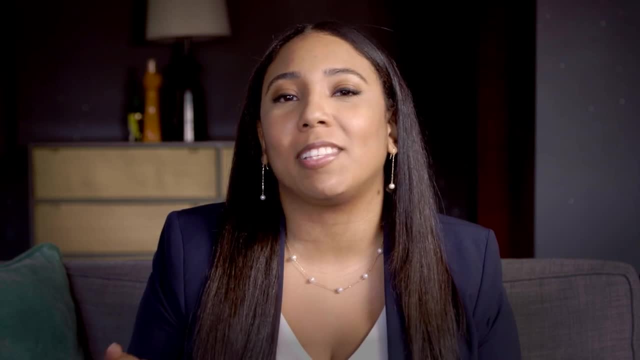 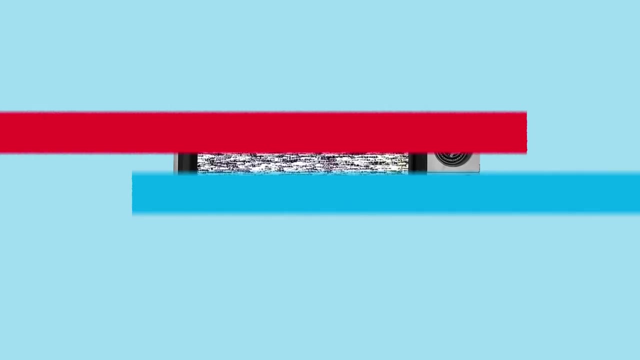 Always wear sunscreen. Eat a balanced diet. A penny saved is a penny earned. You probably all learned these lessons as a kid, maybe from your parents or, if you grew up in the 80s, from the public service announcements at the end of every episode of the GI Joe cartoons. But chances are despite. 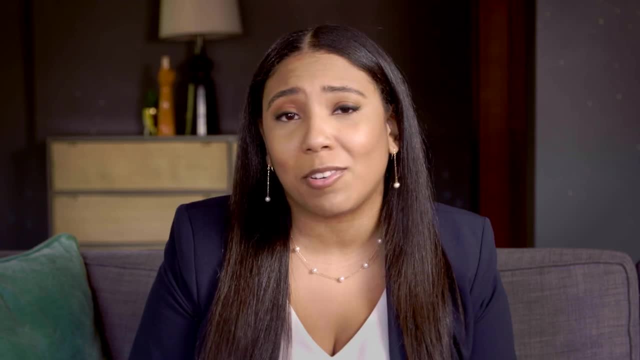 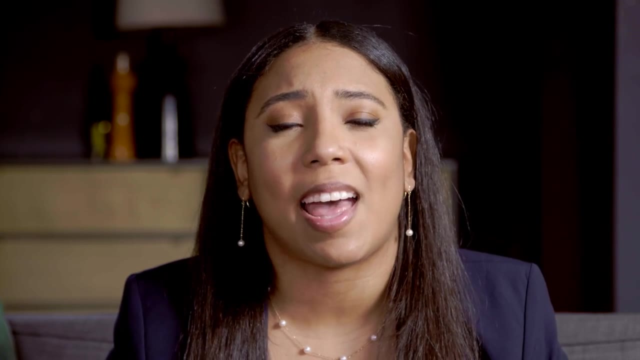 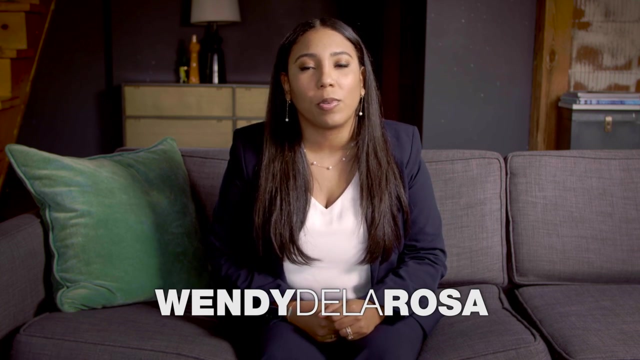 knowing this, you still stepped outside without putting on sunscreen, devoured an entire bag of chips in one go or spent way more of your paycheck than you anticipated. So why is that? A few years ago, two Yale professors coined the term GI Joe fallacy to describe this very 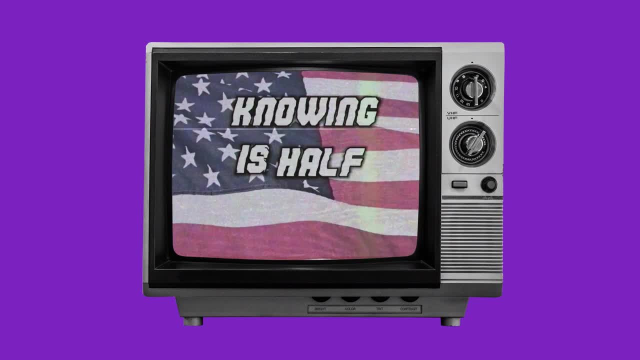 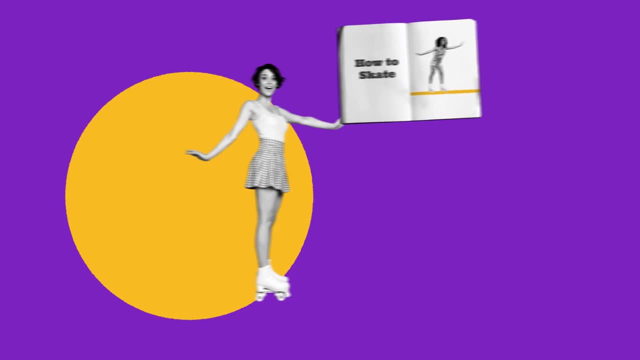 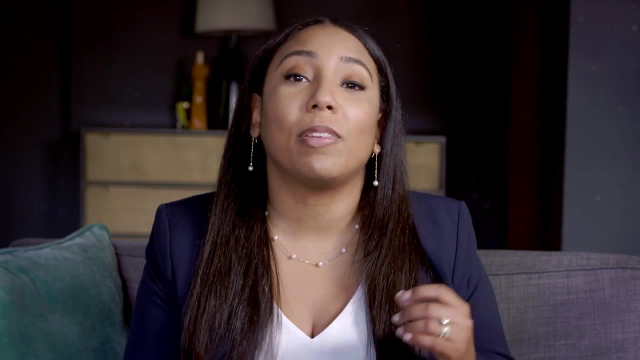 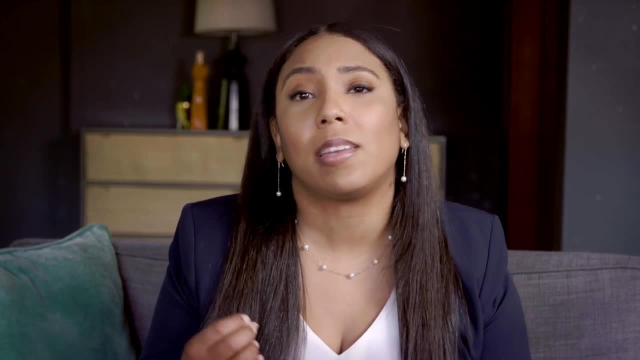 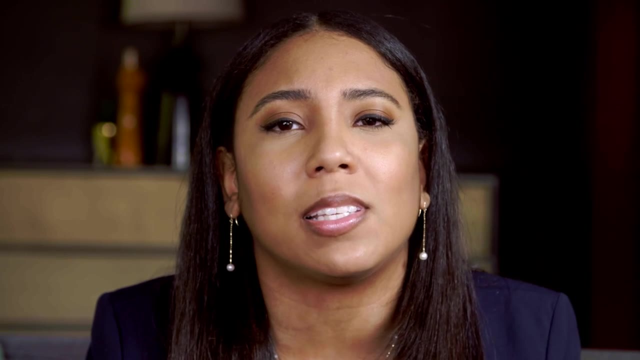 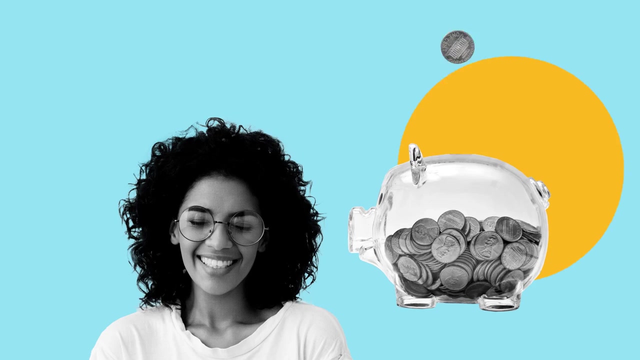 to save money to cut back on their expenses or to manage their debt, even after they've taken a financial literacy class, And the reality is that people fundamentally know what they need to do to improve their financial situation. We all do. The equation is simple: They need to save more. 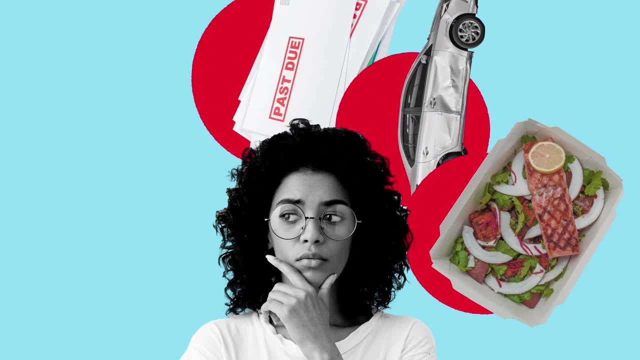 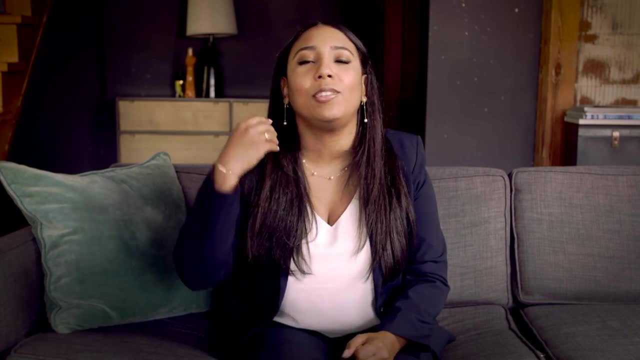 and spend less. But the thing is that's just really hard to do. It's easier said than done, And I've been in this boat as well. So, for example, I had a magazine subscription that I knew I should just cancel. I never read the magazine And every month money was coming out of my 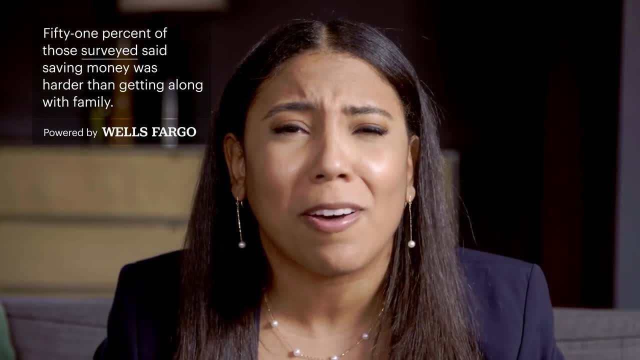 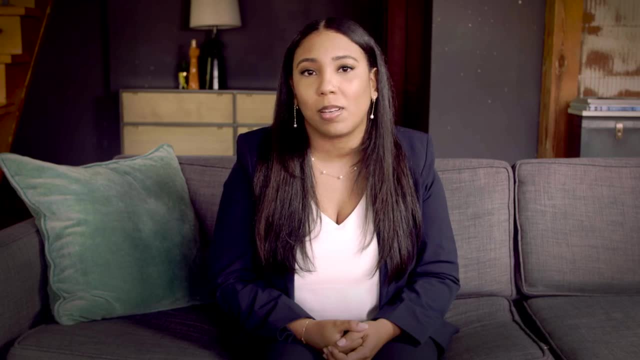 checking account And every time I reviewed my budget I saw it. I knew I had to cancel it, but I didn't. It took me two years to cancel that magazine subscription And I'm sure I'm not alone. You probably have some type of subscription that you know you should cancel. 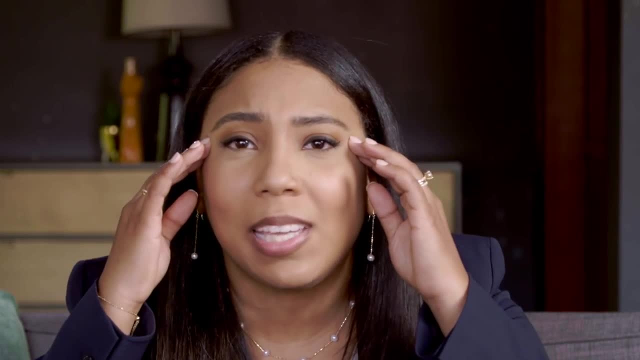 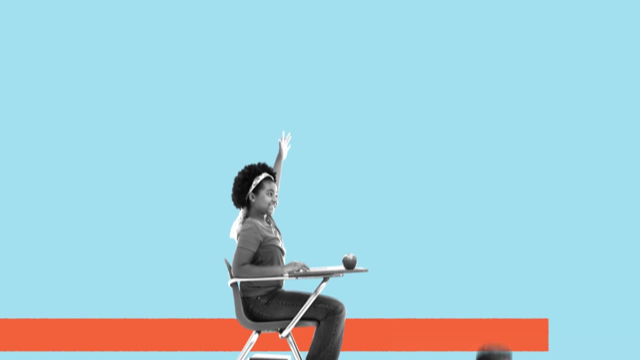 And so the critical piece in all of this is to get rid of this belief that financial security is just a problem that we can teach away. In the US, for example, we spend nearly $700 million every year on financial education programs, Yet a team of